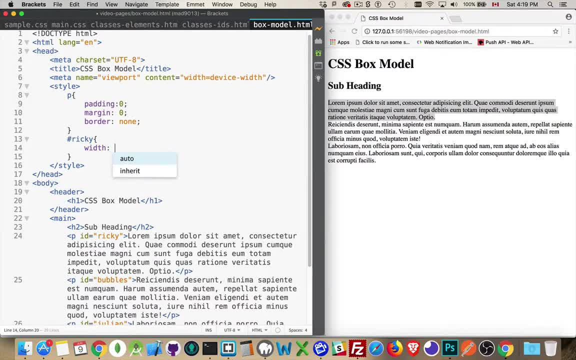 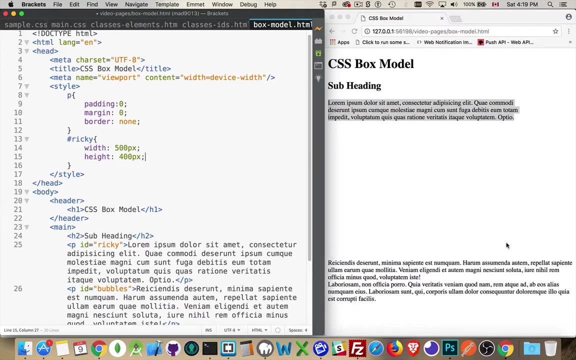 and I say the width of Ricky is going to be 500 pixels. 500 pixels- we'll cut it off here if I say the height of Ricky is going to be 400 pixels. so now I've got 400 pixels tall by 500 pixels wide. that is the size of this element if I shrink it down. a. 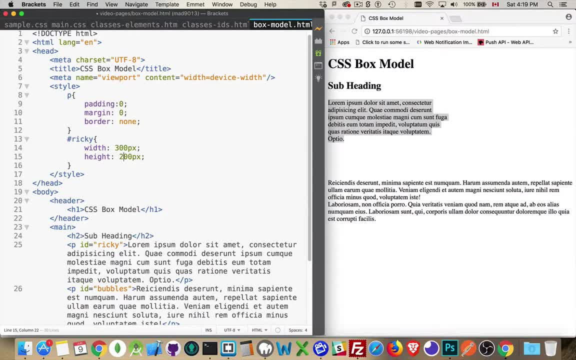 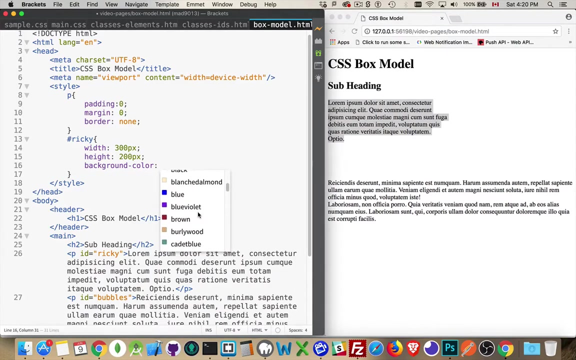 little bit. let's say it's 300 by 200. that is the size of it, so that blue area when I click on it. that is the 300 by 200. that is the content area if you give an element a background color. so let's say it's going to be Burley wood there. 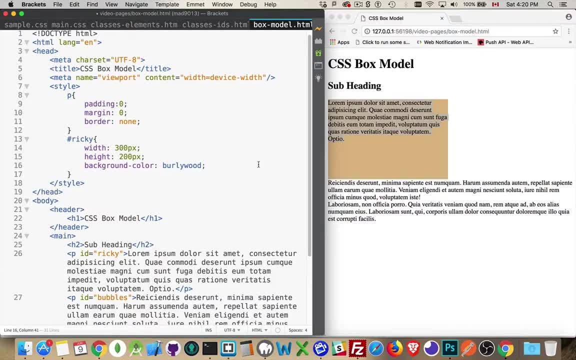 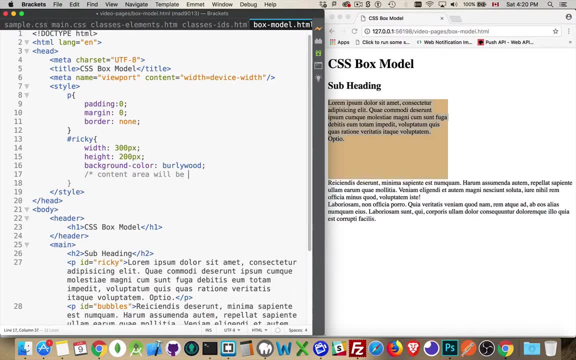 we are. that is the background color for the content area. put a comment in here. content area will be Burley wood. that is the first layer of the box model. now, outside of this content area, there is a layer of padding that you can put on. right now it's zero, so zero pixels on. 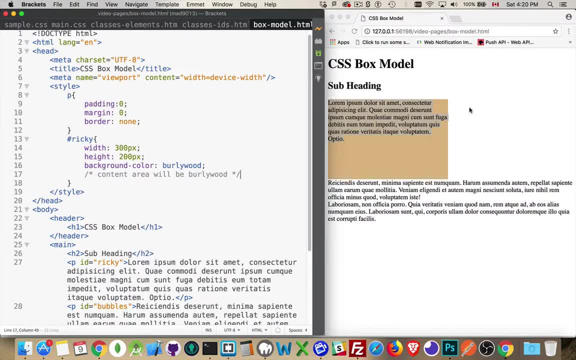 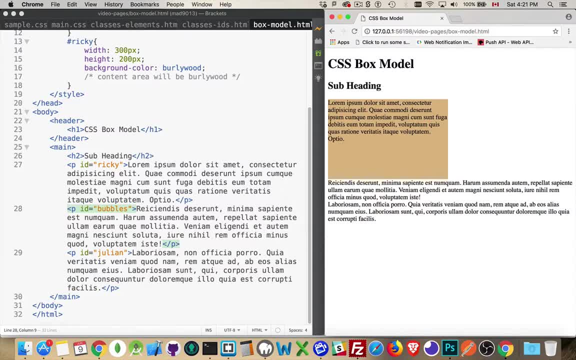 browser. here you notice how this text is pressed right against this edge. here there's no space between the edge of the text and then again at the top. it's right against the top. I mean there's a little tiny bit of line height in there, but really the text is. 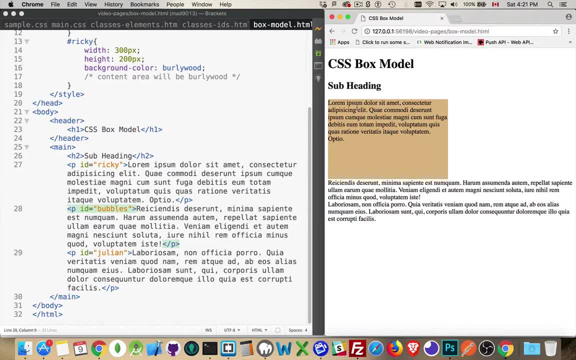 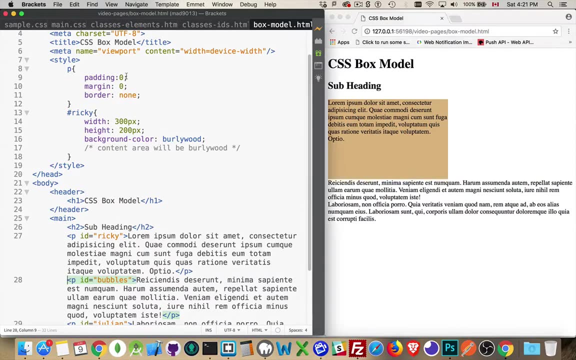 against the top and it's against the side. This is never a good idea for your design. You never want to have the text touching the border or the text touching the background color change anywhere. So padding- this is how we create the next layer. 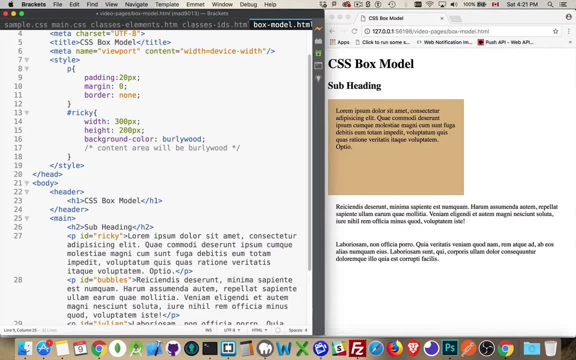 If I said that padding is going to be 20 pixels, I now get 20 pixels on the top, bottom, left and right. All four sides are getting 20 pixels. I've created some space And the background color of the padding. 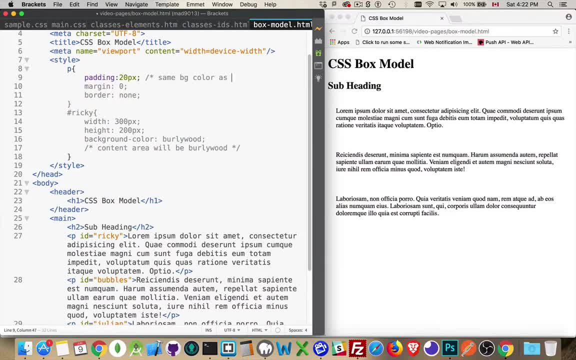 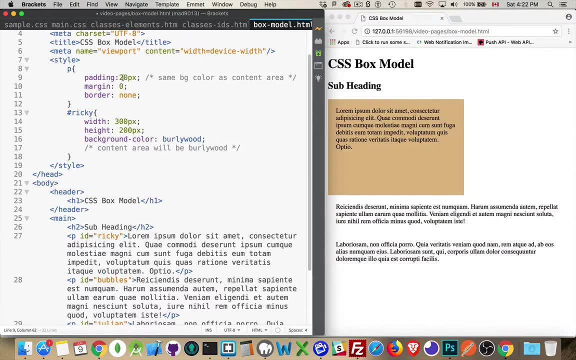 same BG color as content area. Important to remember that That's one of the big distinctions. So padding, border margin, they're all just extra layers of space around the content area. The differences between them really have to do with the colors. So padding automatically gets. 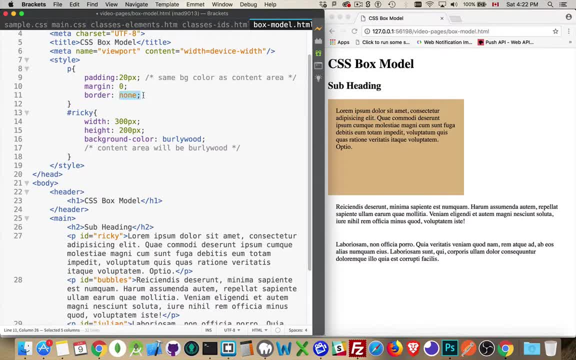 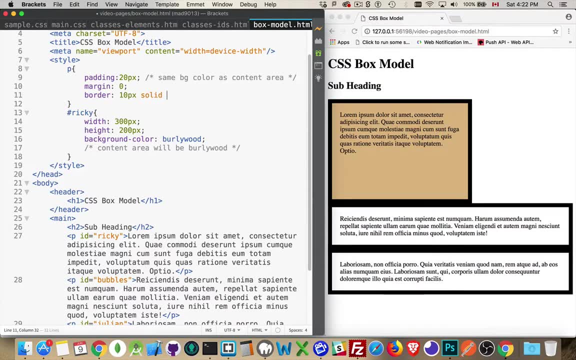 whatever your background color is. Beyond that we have a border. So if I said I wanted 10 pixels solid, by default it's black. Let's go with something that's not going to look nice with this red. Okay, all three paragraphs are getting 10 pixels of padding. 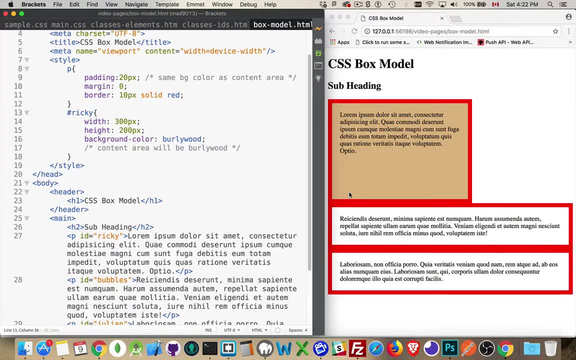 and then, or sorry, 20 pixels of padding and then 10 pixels of border, So 20 pixels around here. So in between the content area and the border there's 20 pixels And then the border is 10 pixels wide. 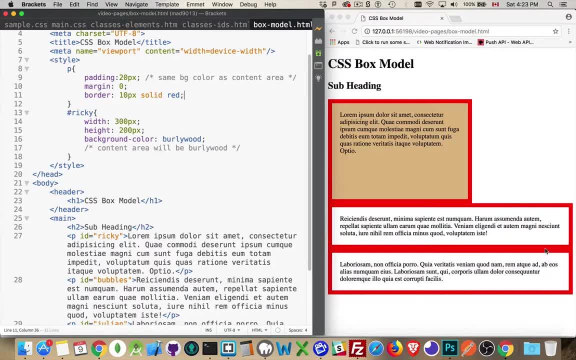 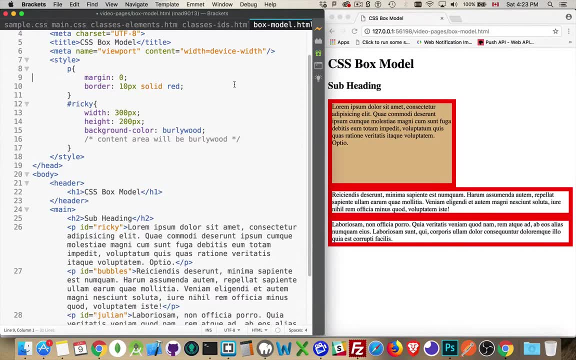 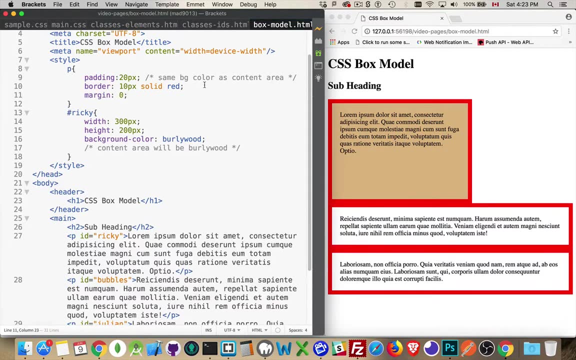 So 10 pixels of the each of the four sides, 20 pixels on each of the four sides and then margin. That is our last one. Oops, Want to do? cut that and paste it below. There we go. Now it's in the order. 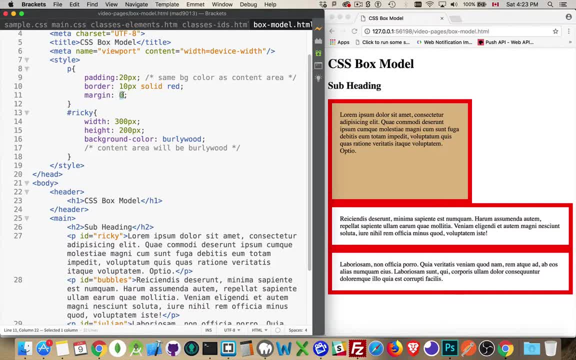 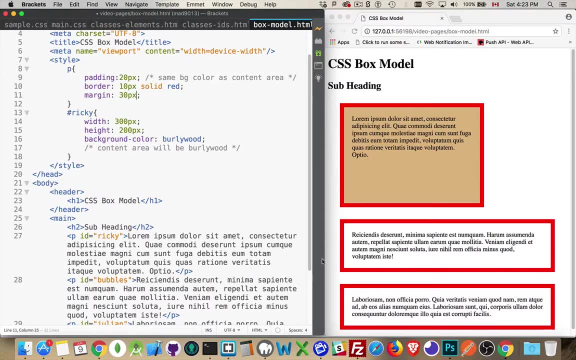 Padding border margin. That's the order that it gets applied. If I add 30 pixels of margin, there we are. I have 30 pixels of margin on all four sides. Now it doesn't look here like: this is 60 and this is 60.. 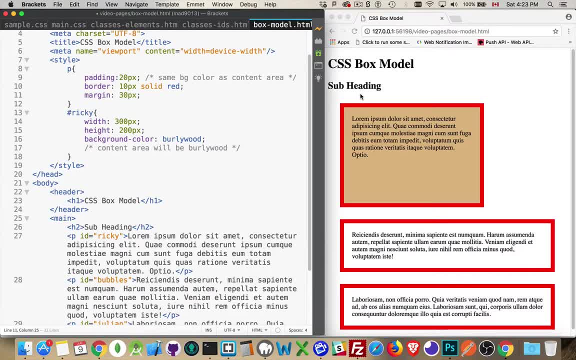 There's a gap here which is really only just a little bit more than 30 pixels. So what's going on here? Whenever margin overlaps with margin from another element on the top and the bottom, the largest size of the two is what gets applied. 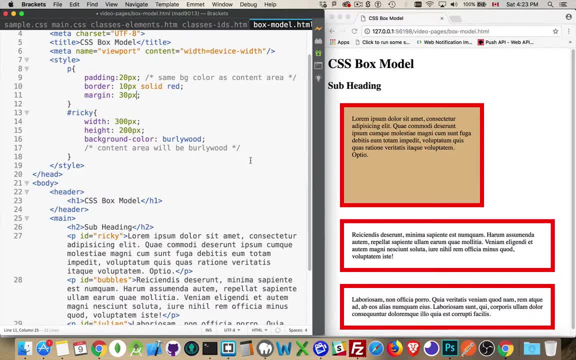 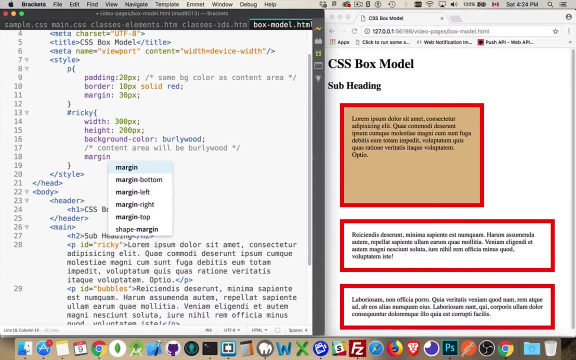 So they're both 30 pixels. 30 pixels is what's going to be applied. If I said that, Ricky, my first paragraph was going to have margin on the bottom of 50 pixels, then what's going to happen is this space is going to become 50 pixels. 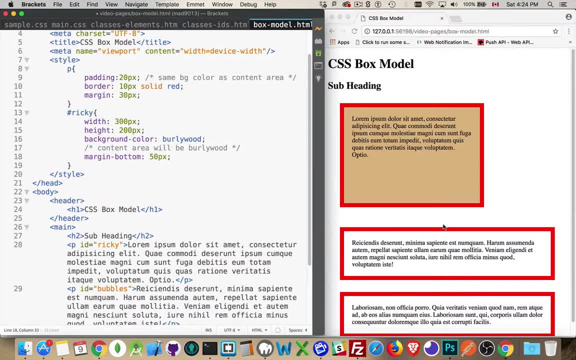 There Now. this is 50.. This is 30. Doesn't matter which one I did. The larger of the two values is going to win out. This middle paragraph has 20 pixels. This one has 50 pixels. 50 is the bigger number. 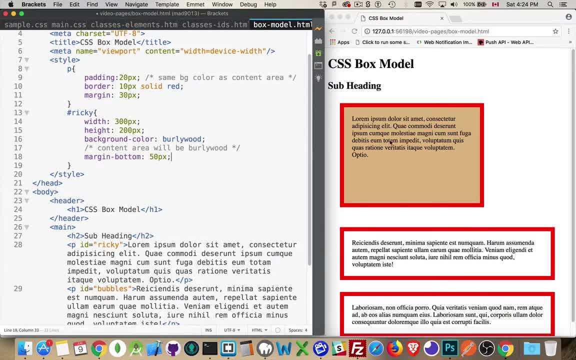 That's what gets applied Left and right. both will be applied. So if there was another paragraph sitting here beside it, they would each have their 20 pixels- or sorry, 30 pixels of margin, So there'd be a total of 60 between the two of them. 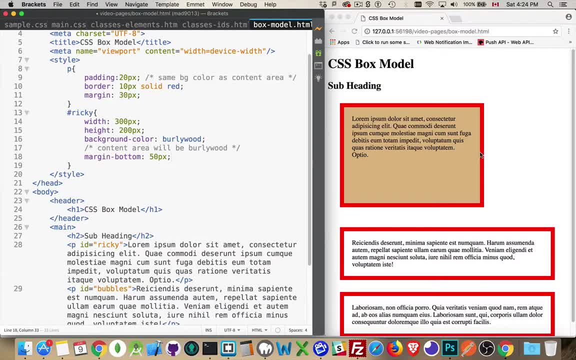 All right, Padding border margin. I was saying before that color was the biggest difference between them. Border: You specify the color Padding. It's only going to be a little bit more than that, So I'm going to go ahead and do that. 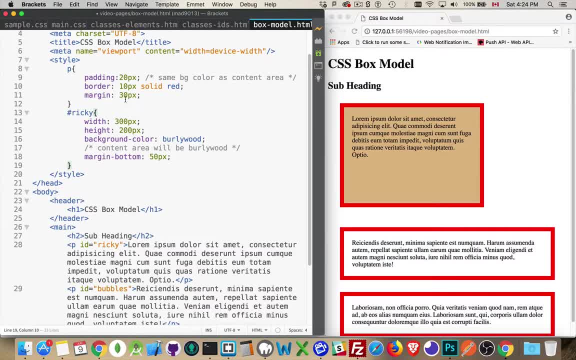 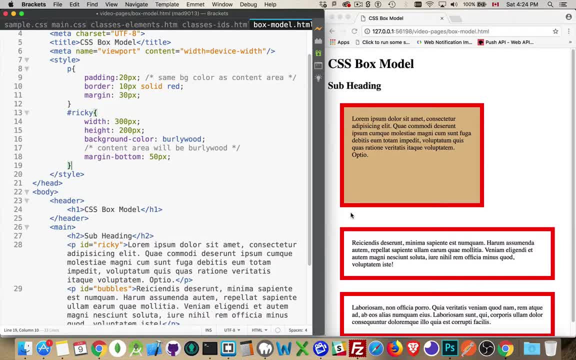 I was saying before that color was the biggest difference between them. Border: You specify the color Padding, It's automatically the same as the background Margin is always transparent. There we are. That's the difference between the three of them. Padding border margin. 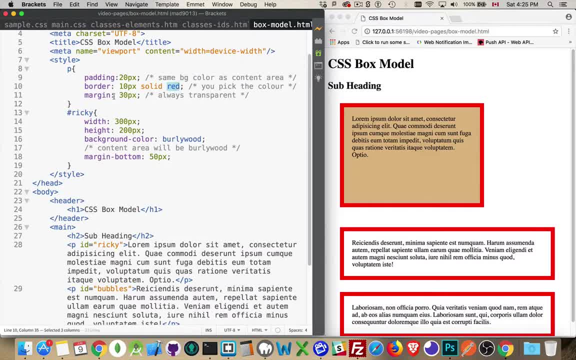 Padding, It's the same as the background Border. It's always transparent. You choose Margin, Always transparent. The three of them really are just three more layers of space that are added on top of the content area. The content area, that's your height and your width. 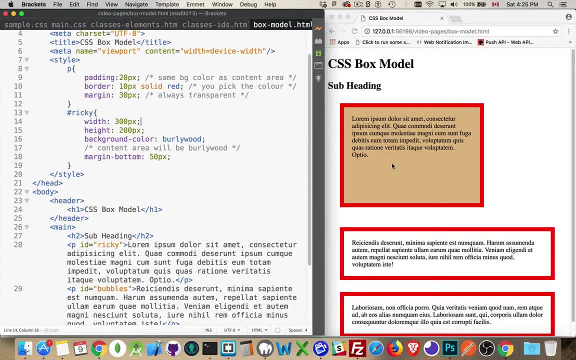 Going beyond that. that's your padding border margin, And it's up to you to decide which ones you want to use. If you're not setting color on any of them, it doesn't really matter which one you're using most of the time. 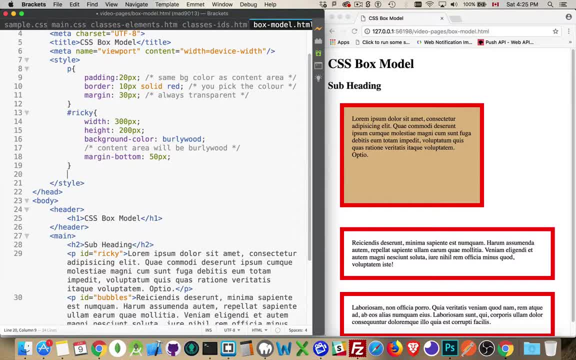 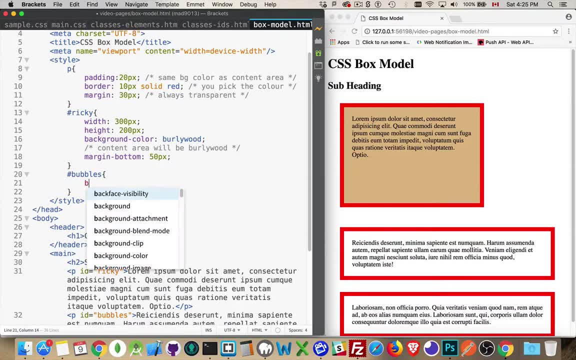 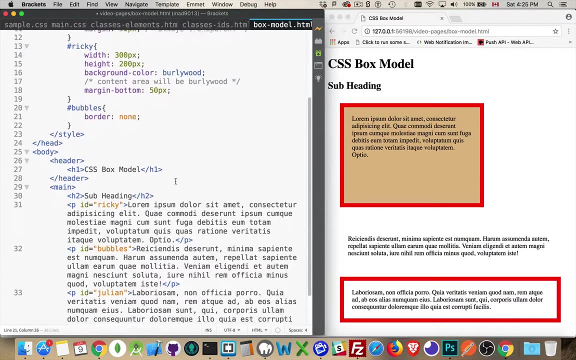 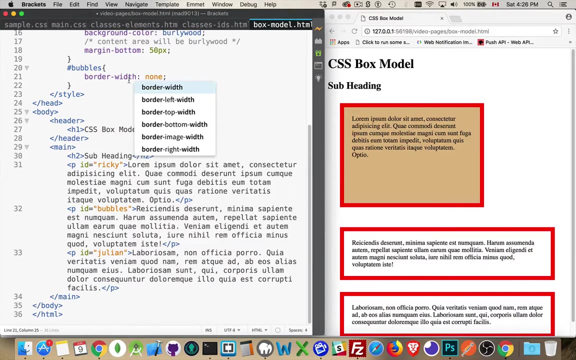 So we can come in here and we can change bubbles or julian Our other two paragraphs. We can say that border is set to none, Or we can say zero as the value. So border width is zero. That gets rid of it as well. 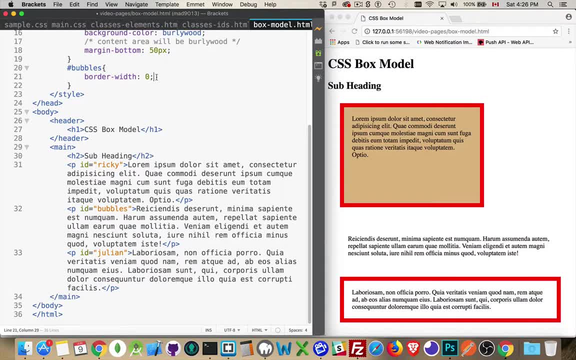 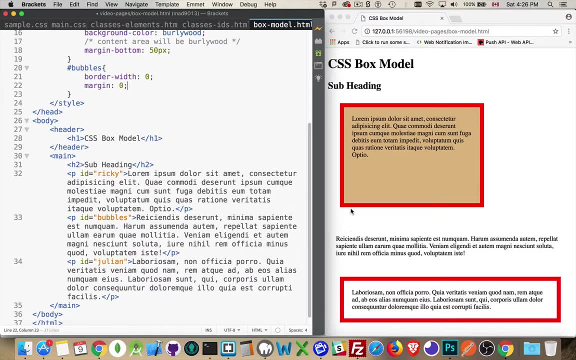 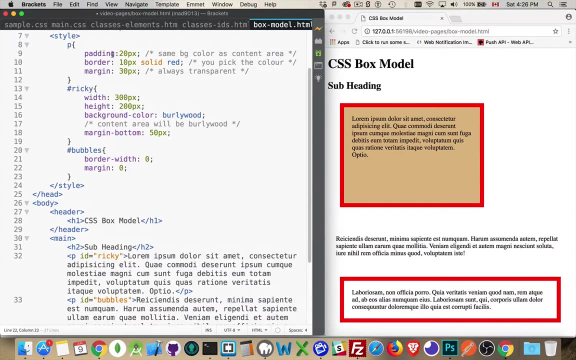 So that got rid of the 10 pixels that we had for that And margin we can set to zero. We still get the big space up above here This is the 50 pixels And down here there's still 30 pixels And we still have our padding of 20 pixels around. 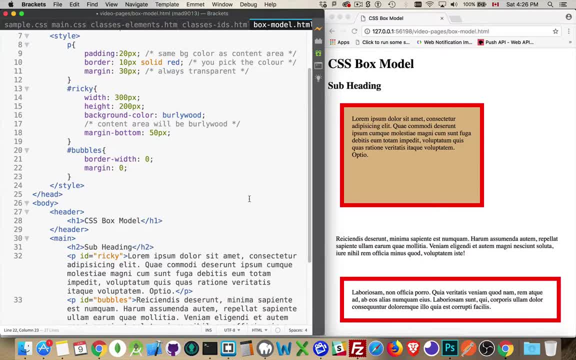 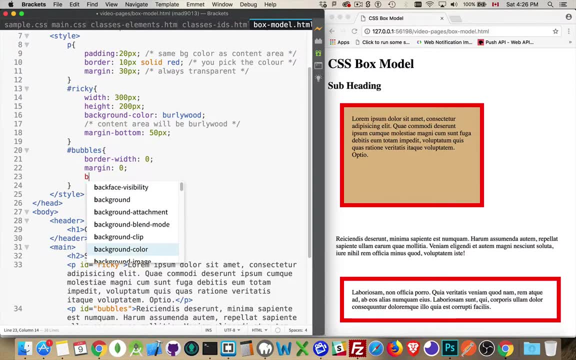 We just don't notice it because it's the same as the page's background. It's that transparent color which shows the white background of the page. So if I were to add background color, Let's go with cornflower blue. There we are. 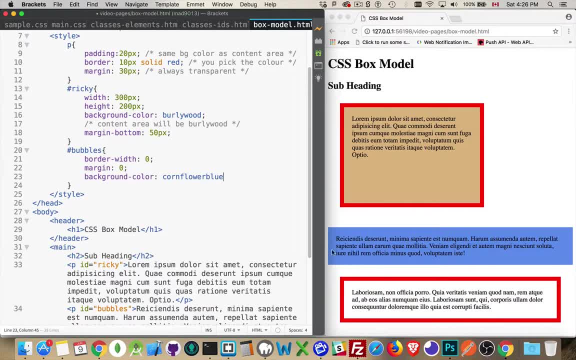 Now I can see that there is space around here Where the background doesn't have text on it, So this is padding. There is no border. We set the border width to zero, So there's no border And margin has been set to zero. 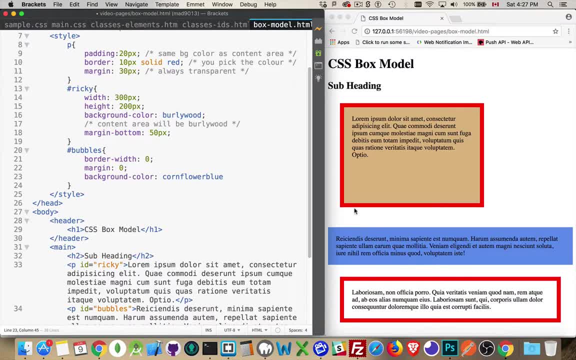 But there's still space. There's still 30 pixels here And 50 pixels here. 50 pixels was set as the margin box, The bottom on this one, And 30 was the default right here that we set on all paragraphs. 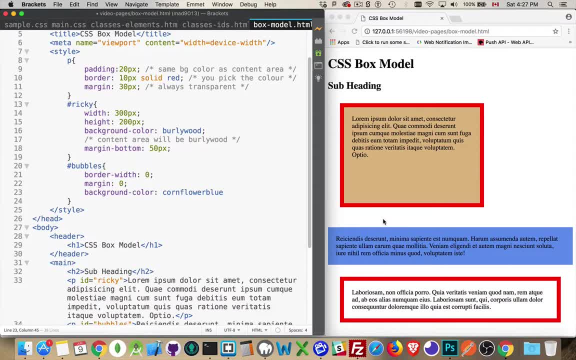 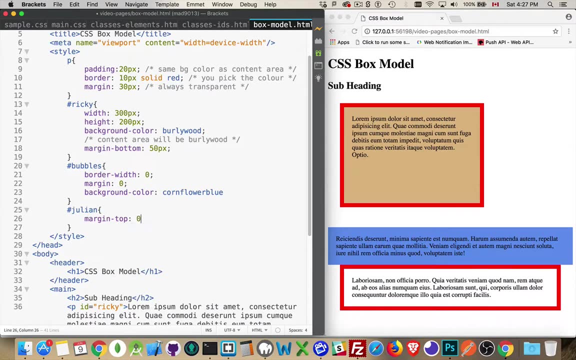 So this guy's got 30 on the top, This guy's got 50 on the bottom And that is the gap that we have above and below. If we were to target that third paragraph And set margin top to zero, You'd see all of that space disappear. 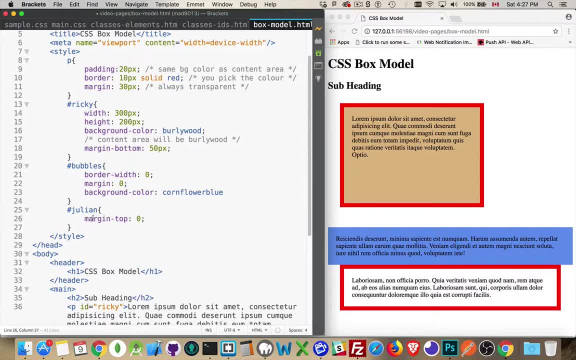 That was the only thing holding it apart Was the margin top on here. He had zero, He had 30. The 31 out is the bigger value, So that's why we got it there And that's the fundamentals of the CSS box model. 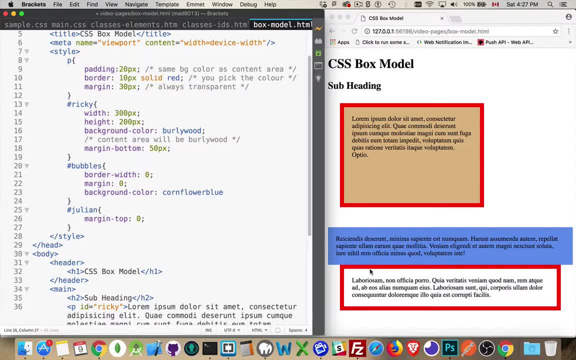 If you understand how the content area has padding border margin layered around outside of it And those three layers exist on every single element, No exceptions. All elements get those three values applied to them Outside of the content area, Then if you understand that,